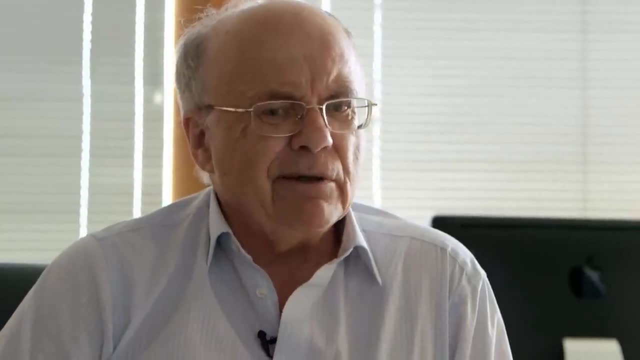 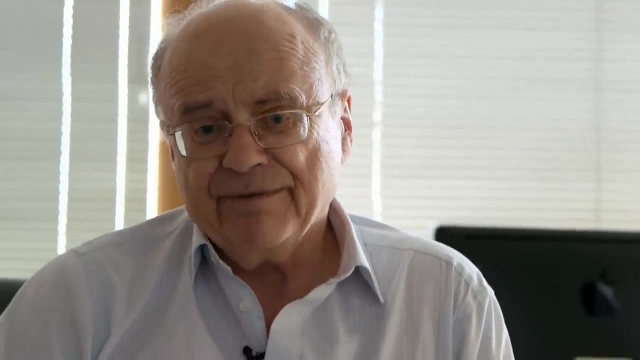 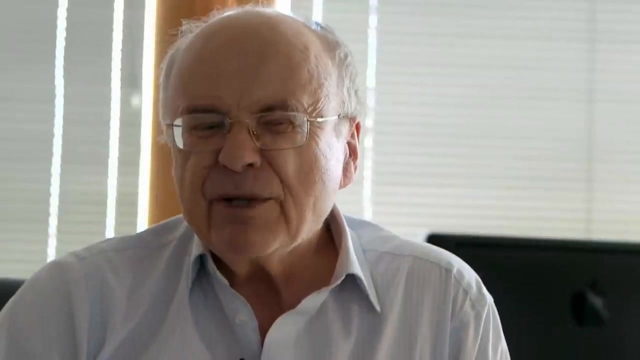 And there would be a great danger in thinking: well, surely you can do anything then in for loops, Why bother with a recursion at all? Well, there are some things which are so fundamentally recursive that you just have to do them recursively. It became clear to mathematicians really at the turn of the last century about the nature of functions in general. 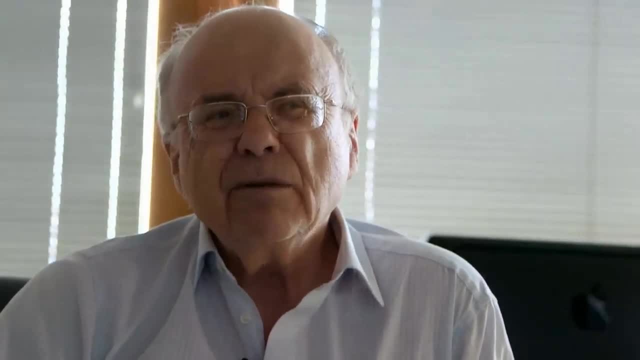 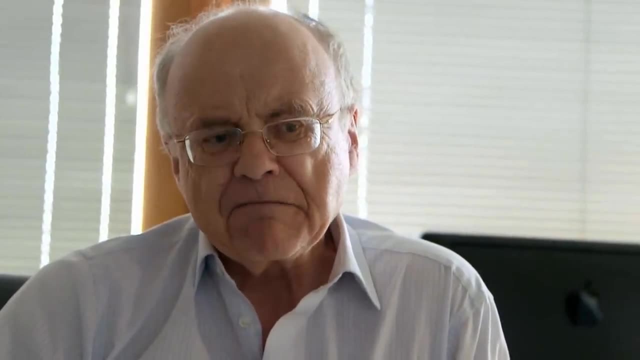 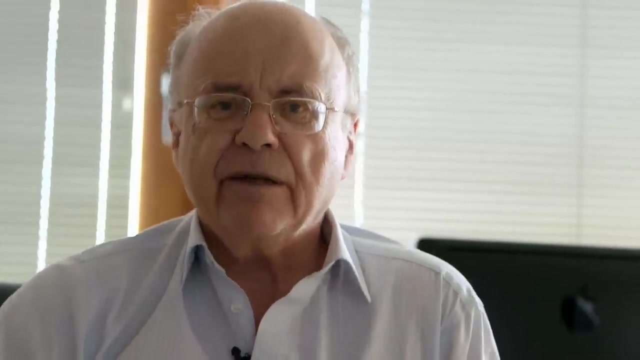 that there were some things that were so, if you like, huge, so enormous, so badly behaved that they just had to be recursively defined, And I think one of the earliest people to realise this was a research student of David Hilbert's. 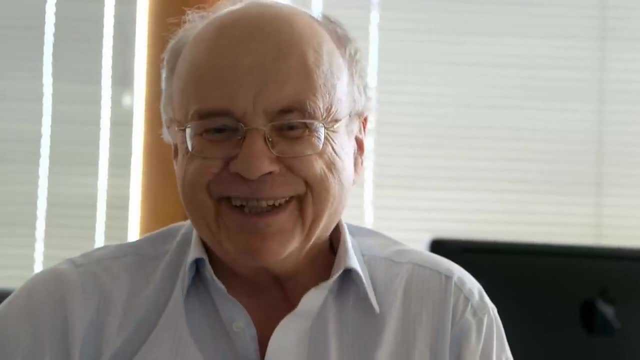 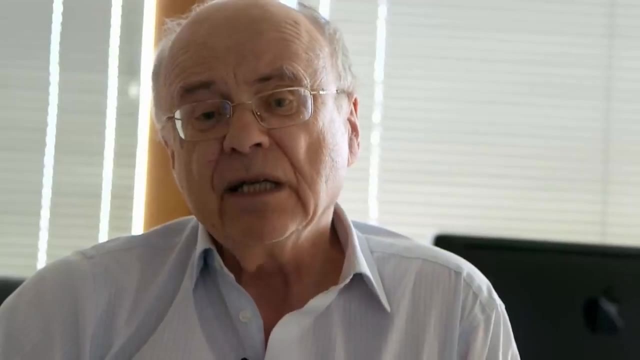 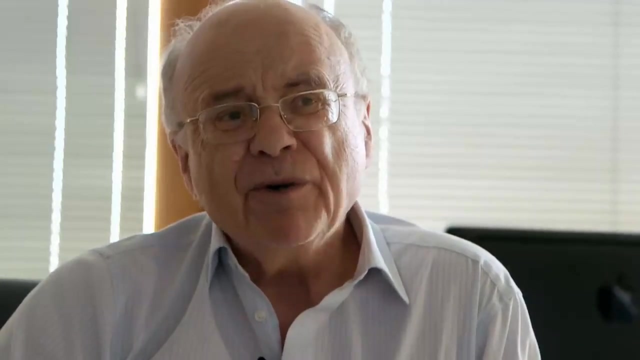 Now who is David Hilbert? We're back on Numberphile territory again- Probably perhaps the greatest mathematician of the late 19th and early 20th century. He was a phenomenal mathematical genius, capabilities and so on. 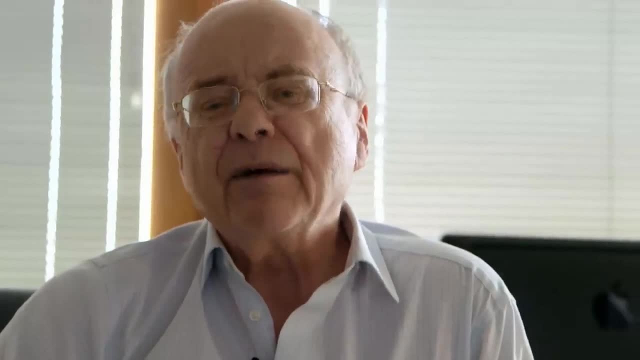 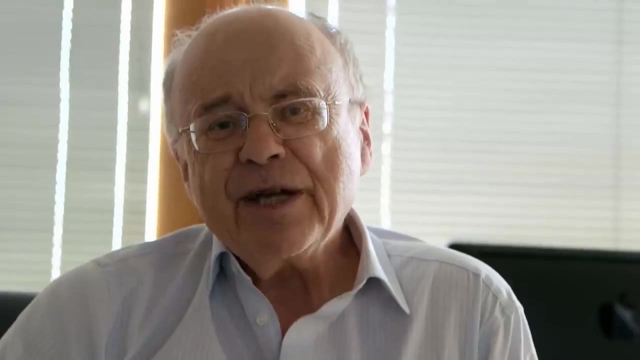 He was at Göttingen in Germany, and I think I'm right in saying that Ackermann was one of his research students, And it's Wilhelm Ackermann's function that we're going to look at today. The test was: can you come up with something that just has to be done totally recursively? 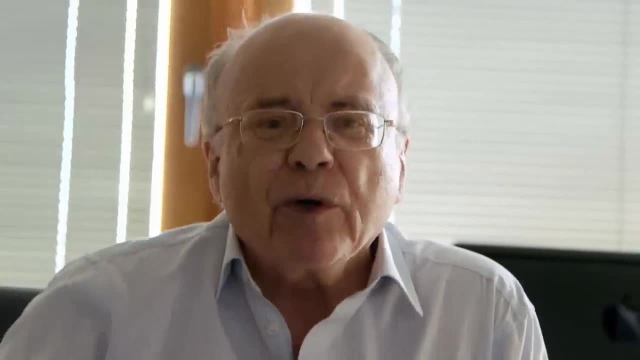 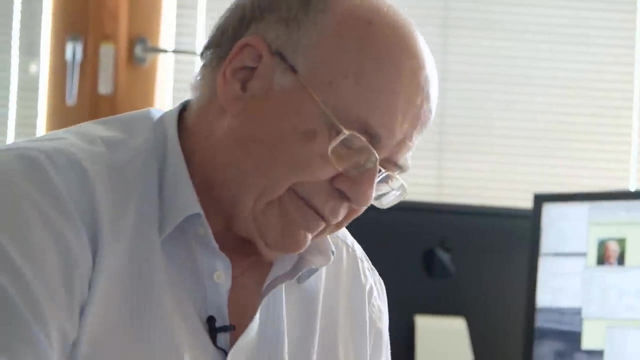 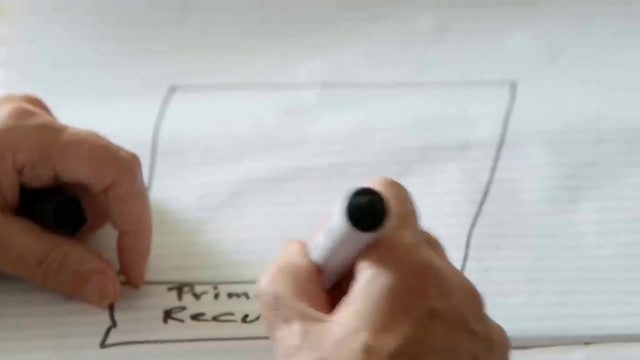 You can't do it, as it were, in a for loop. even though those hadn't been properly invented at that stage, What became clear as a result of work started by Ackermann and by others is that we've got a hierarchy of program types. 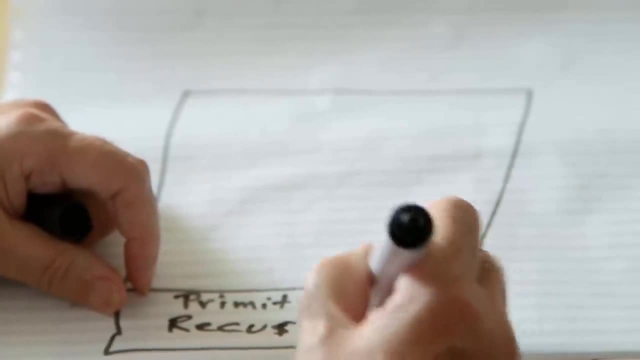 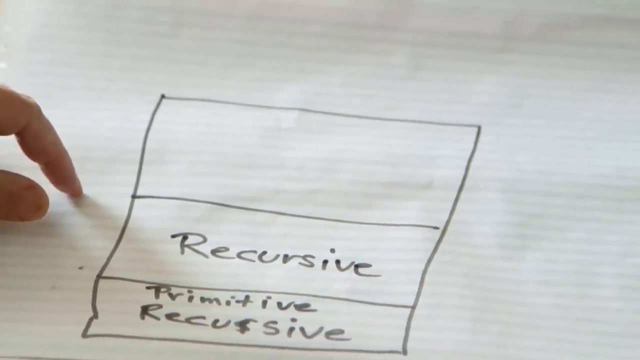 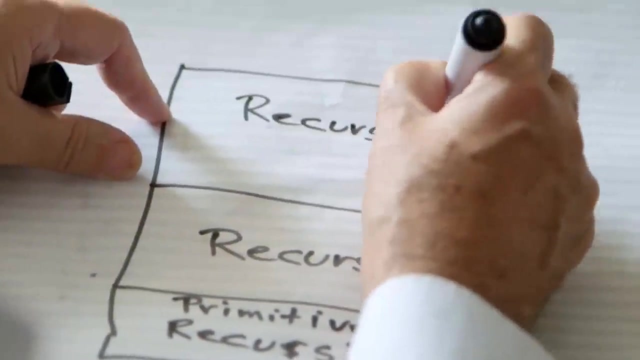 Right down at the bottom, the simple ones we've seen, the ones that can be de-recursed. these are primitive recursive. There's a whole layer on top of that where they're functions, where you just have to define them recursively. Just above this set are the recursively enumerable functions. 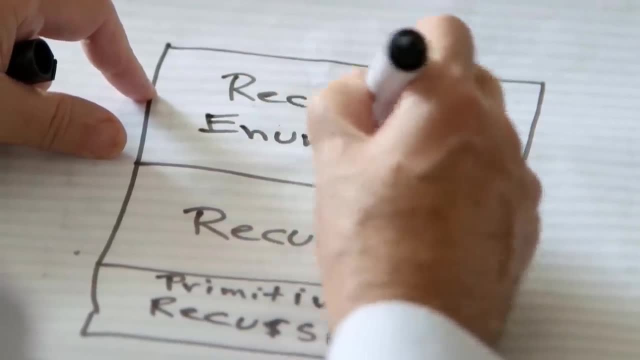 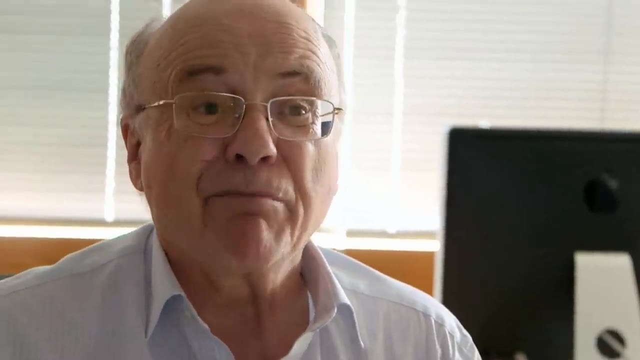 Let's be clear here: By saying primitive recursive, at the bottom I'm including every other program that isn't recursive. I'm regarding a thing that just goes through a sequence as being a very simple example of a primitive recursive program with no real recursion in it. And anything that's got for loops or nested for loops. well, actually you could have done that recursively- And probably languages like Haskell do, for all I know- But they still count as the simplest form of program: Primitive recursion. if it's got recursion in there at all, you could always de-recurse it, make it into for loops. 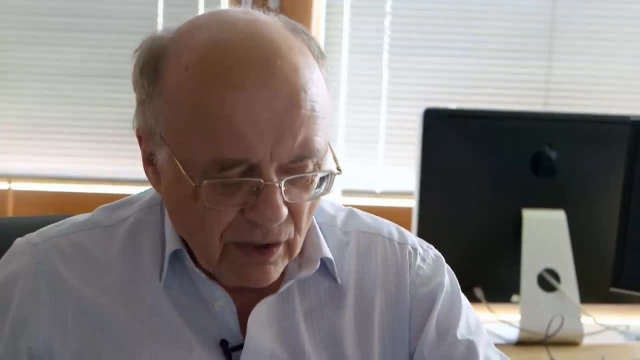 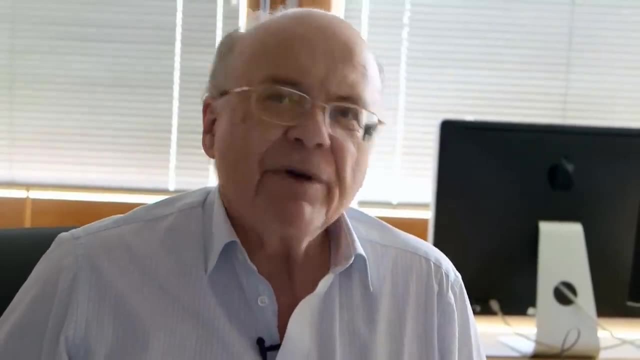 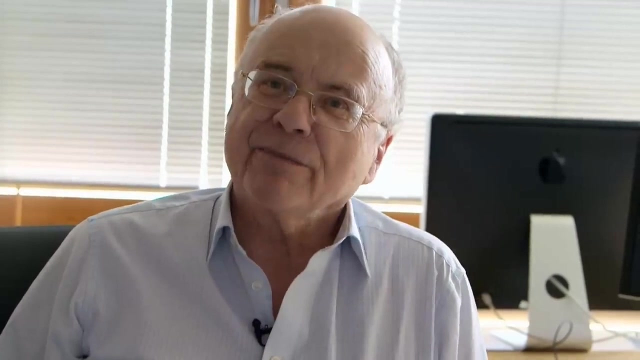 This next thing recursive. on top of that there's an even more problematical set of programs above that which says they're recursive, but for some values of the arguments you put into the function they will stop and give an answer, And for others they will go on forever. 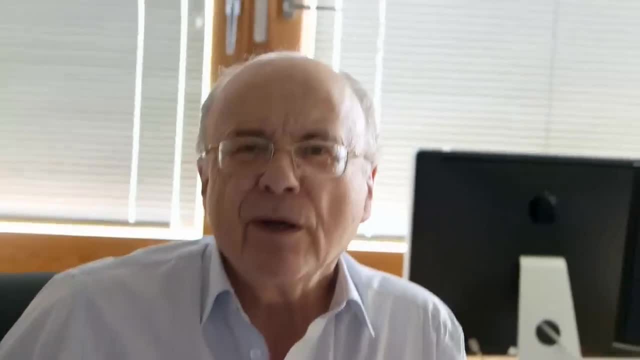 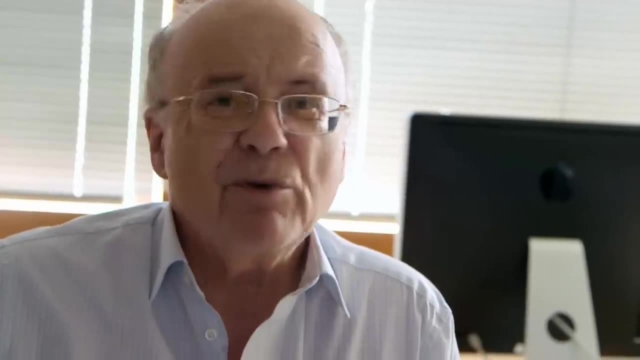 And they will never, ever stop. How do you define forever? then? Go on Forever and ever and ever. They will go into just repeating the same old stack frames- and you may not be aware of it- And just go round and round and round. 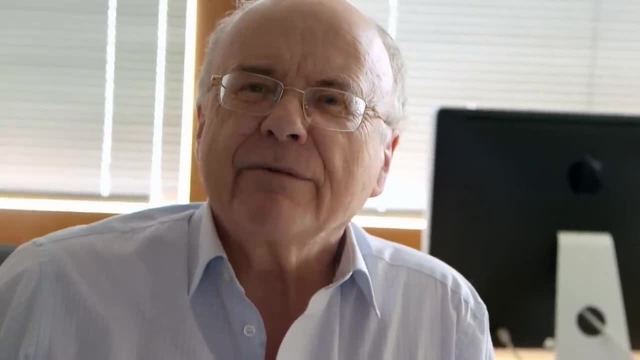 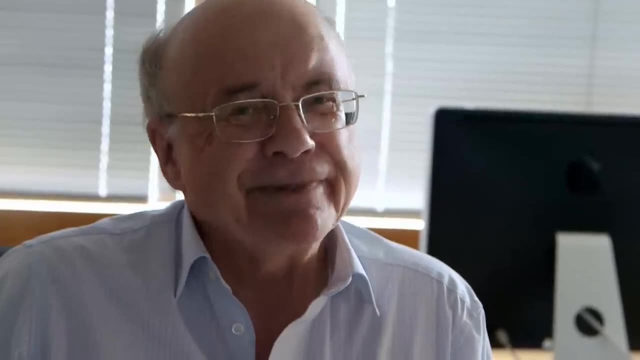 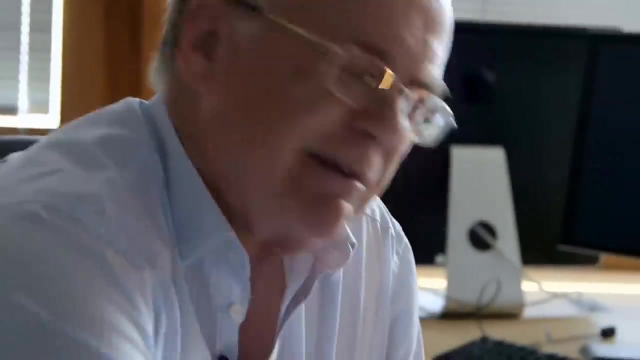 And then you'll say: but how can I decide ahead of time for given arguments whether it will stop or won't? And the answer is: Hello, Alan Turing. In general, that may well be undecidable. So above here out in hyperspace is the great undecidable universe. 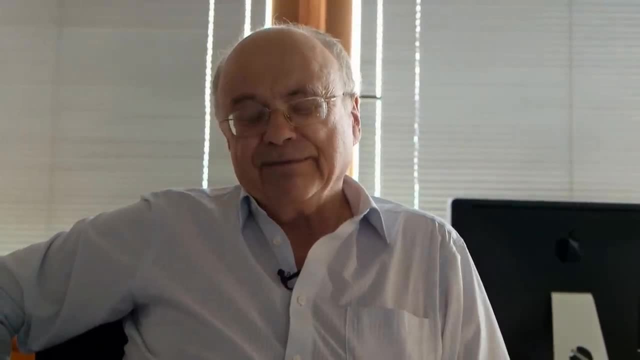 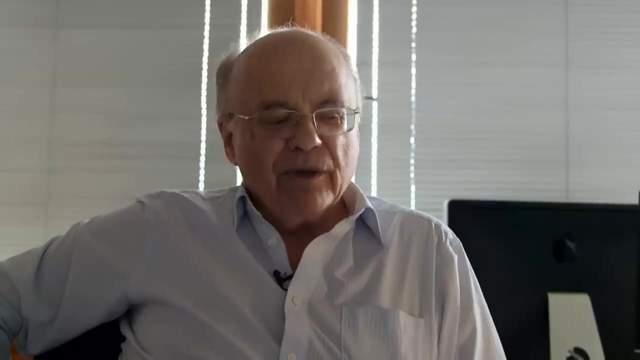 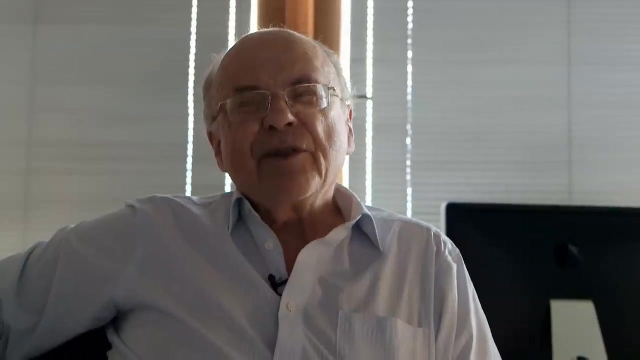 There are some problems you can set in computing that just are not decidable at all, Not by any algorithm, And one of the great names in this was Kurt Gödel in the early 1930s And the second great name for computer scientists. that linked Gödel's work with how computer programs worked. 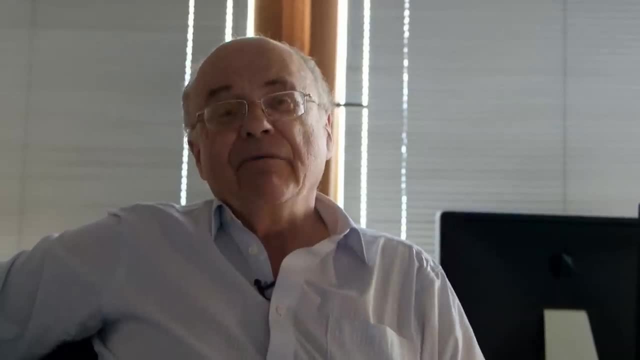 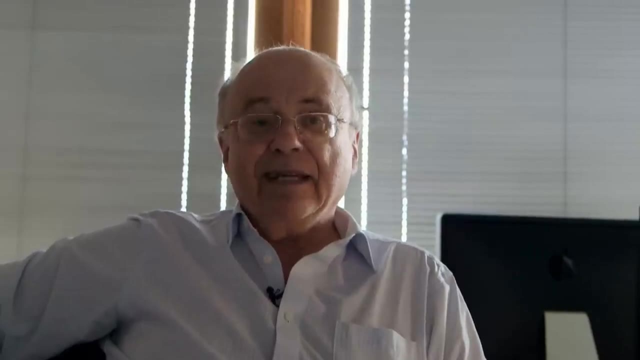 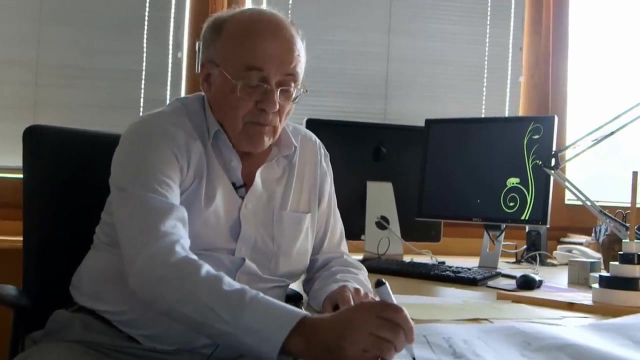 and with his Turing machines was Alan Turing. He wrote a famous paper in 1936 about his Turing machines, referred back to Kurt Gödel's work and basically said there are some things in computing that are undecidable. But for the moment we're coming in here at the next level above primitive recursive. 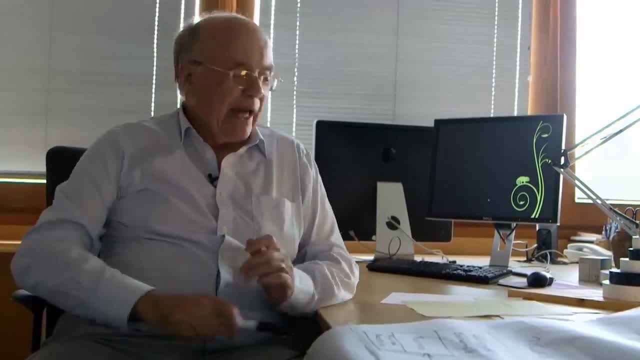 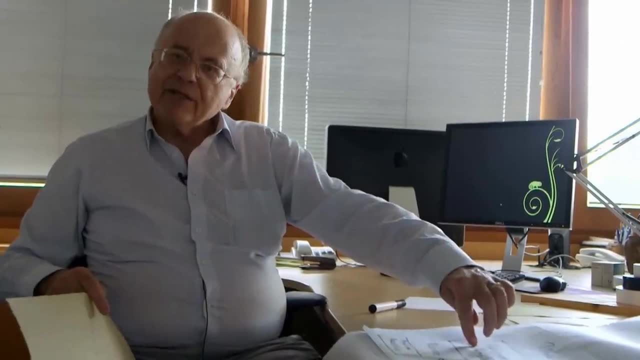 We're going to take a look at a recursive function where I can reason through with you that it will give an answer. It's not in the nasty set above it, the recursively enumerables, where sometimes it would go wrong and just end up spinning and not doing anything useful. 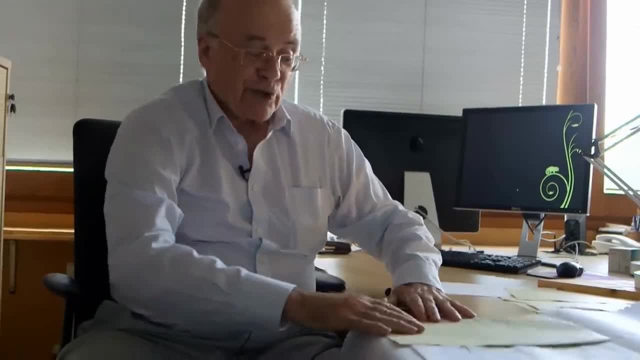 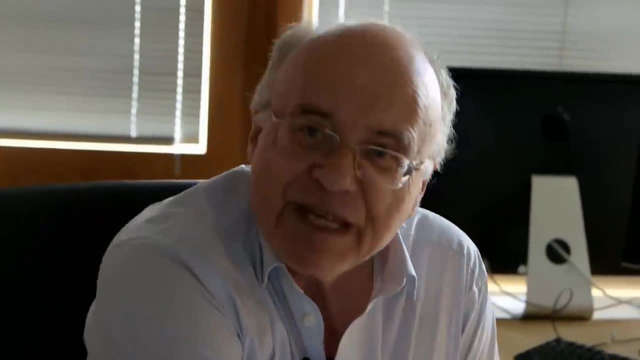 This thing, and this is a good introduction as well to the way that theoretical computer scientists- of which I am not one, but I'll try and give you the flavour about how you can reason about programs and how they behave even without actually executing them. 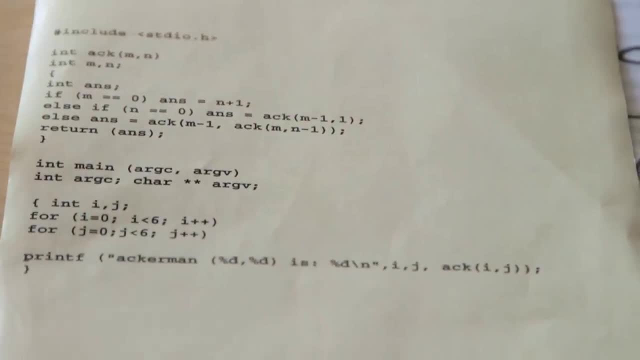 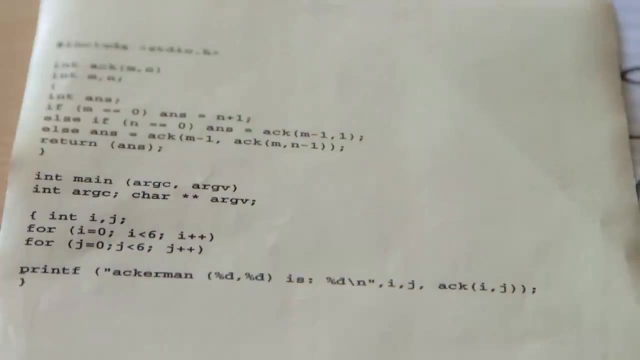 The version of Ackermann's function that tends to be used nowadays, the one modified by Peter and by Robinson. here is where all the hard work occurs. This is the recursive function itself. We declare Ack, for short, a function with two incoming integer arguments. 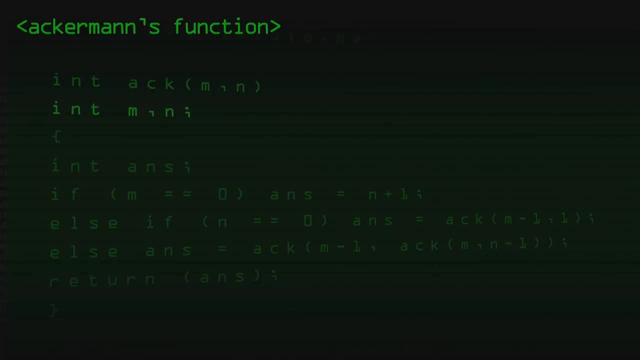 And here, look, it delivers back an integer result. It delivers back the integer result in its local variable that it declares for itself for holding the answer. And eventually, of course, look, it's going to return the answer. But how does it do its recursive horrors? 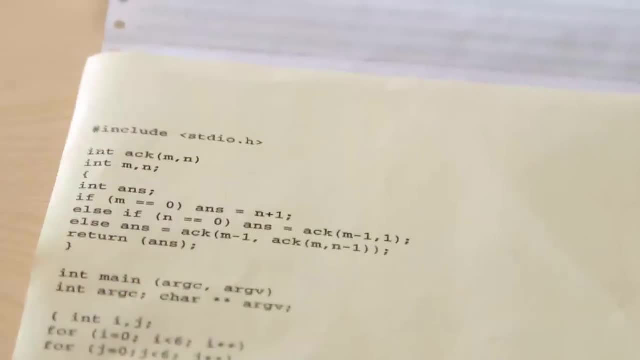 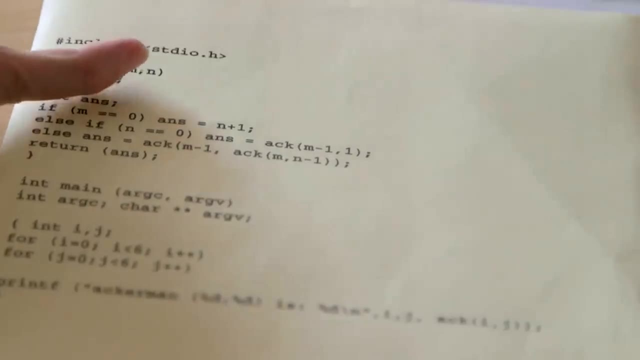 If the incoming argument m is 0, then deliver back the integer answer n plus 1.. So if I came in with Ackermann 0, 2, because the m is 0, it would deliver back 2 plus 1, 3.. 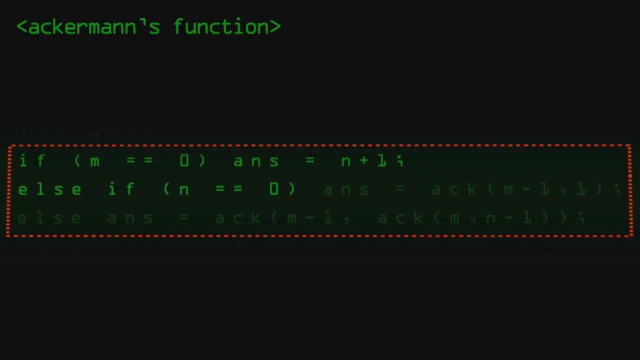 Easy. Otherwise, if that isn't true, if m isn't 0,, if it's any other integer result, else if n is 0, then the answer is what you get by calling up Ackermann recursively again, but this time by reducing the first argument by 1.. 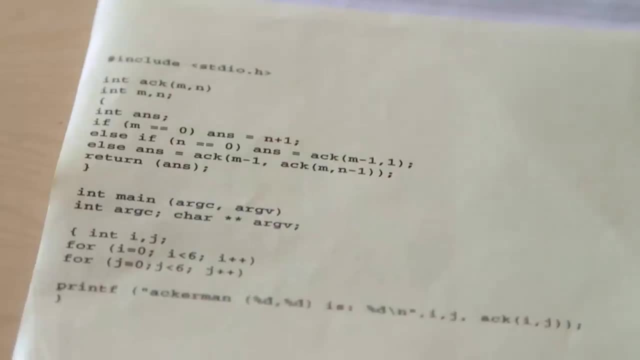 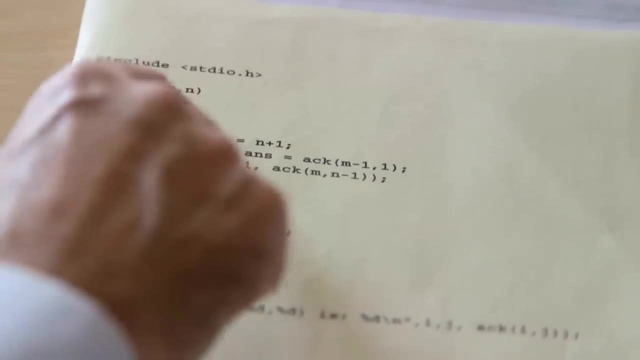 Call up Ackermann with m minus 1, not m, and with the first argument 1.. Otherwise now that's bad enough. Over, here comes the real killer. If m isn't 0 and if n isn't 0, what's the general case? 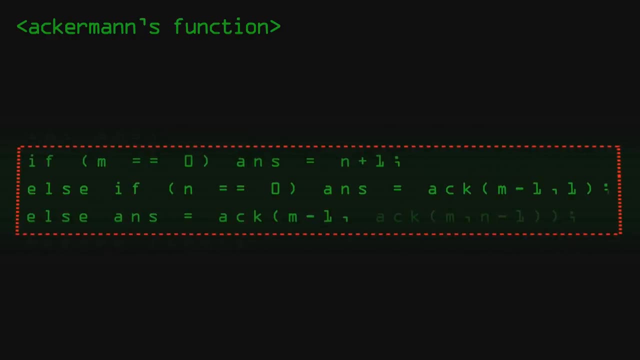 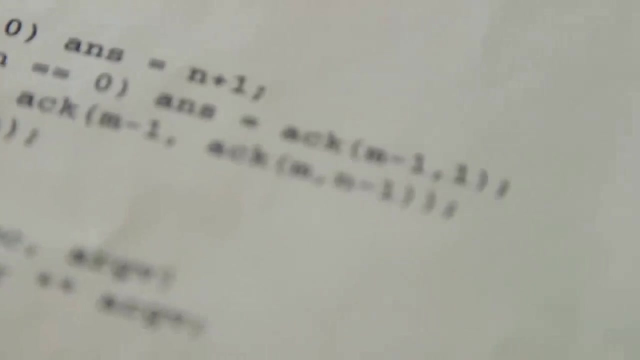 The general case is that the answer is Ackermann of m minus 1.. Notice, you're reducing m again. look, And this is where headaches start to set in. This blows your brain and makes you realise why you can't de-recurse this into iteration. 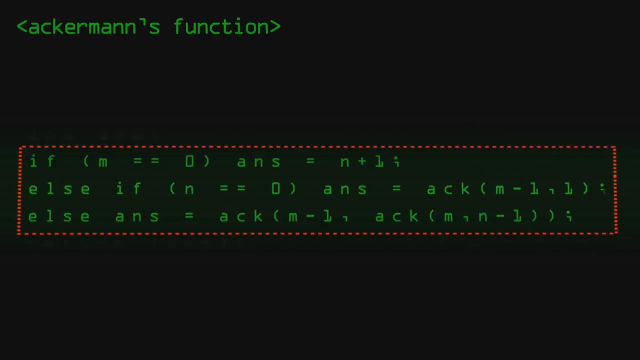 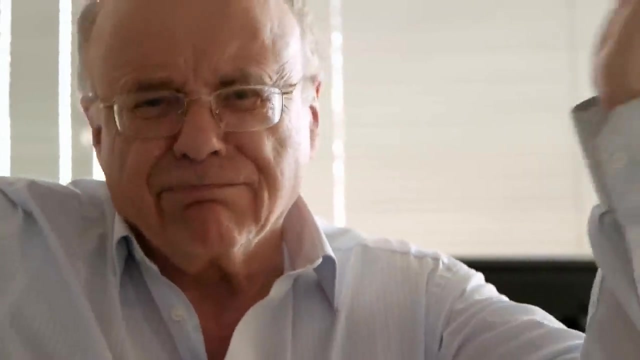 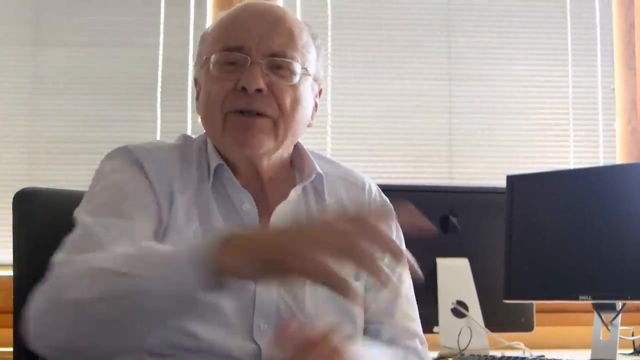 The second argument for that generalised call of Ackermann is itself a call of Ackermann. So you have to go through endless thousands of stack frames to calculate just what the second argument must be to another call of Ackermann: It's going to go through the same agony all over again. 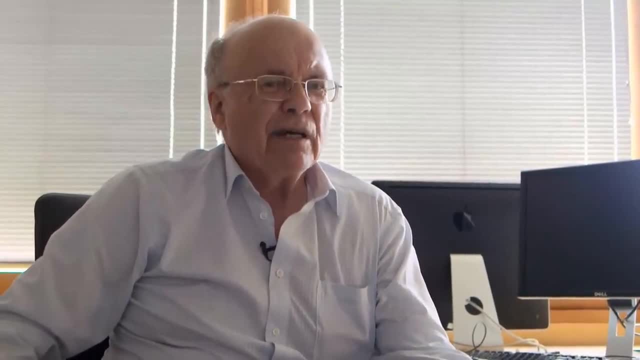 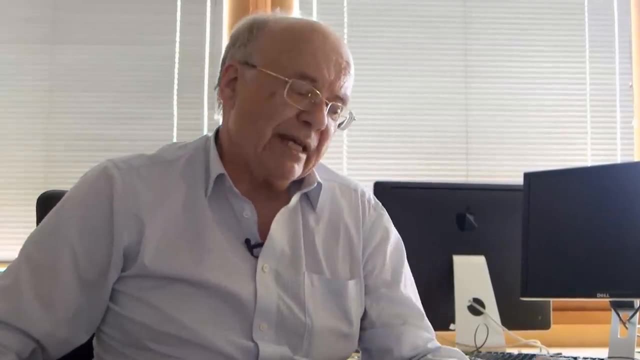 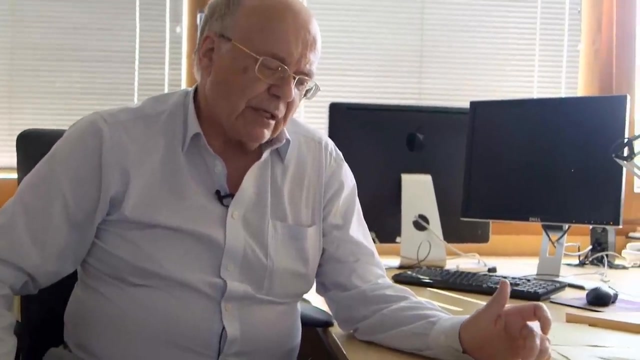 Now I think you can mentally visualise just what a huge amount of computation might be involved here and how big the numbers might get to be. But what I would like to just draw your attention to, because this is important, is that every time m and n are altered, 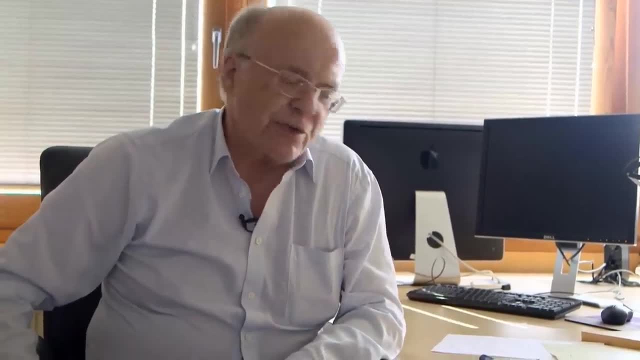 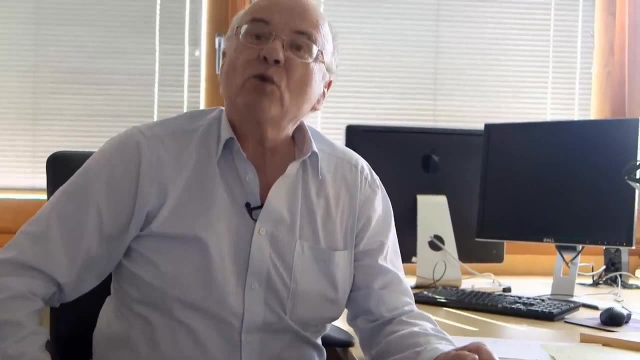 in going round recursively, they reduce. We found out that on the second line it says if n was 0, then you called up a thing with Ackermann in it: Yeah, So you're reducing m at that place. And even in the horrible, worst case. 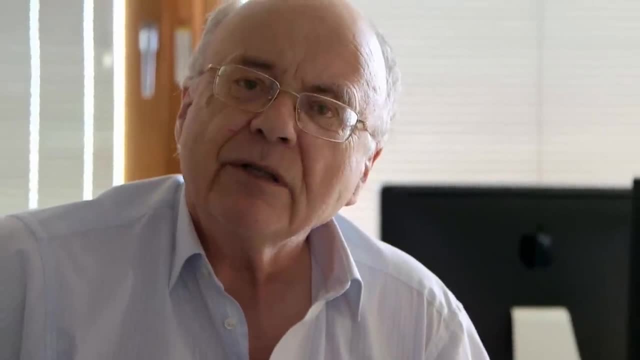 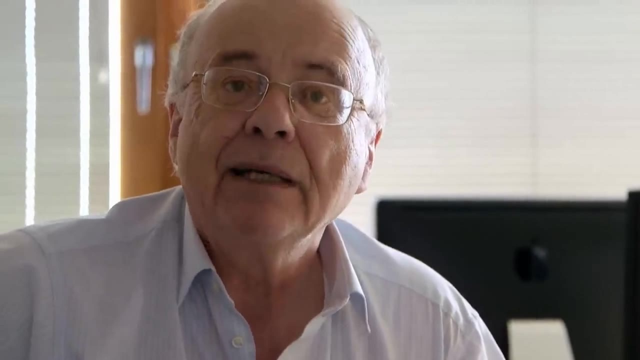 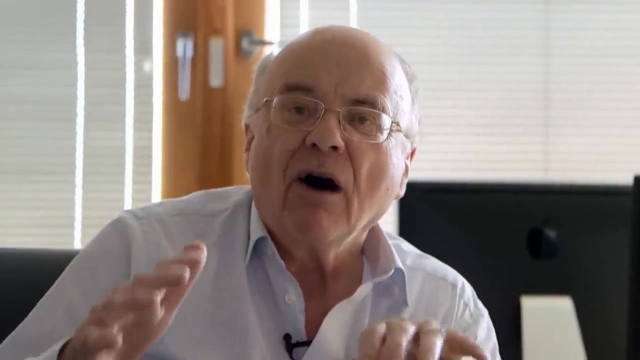 the third line, you reduce the first argument to and within that vile second argument it's Ackermann. So, as you go round this, if m and n change at all, they are reduced. Therefore, if your first two traps, 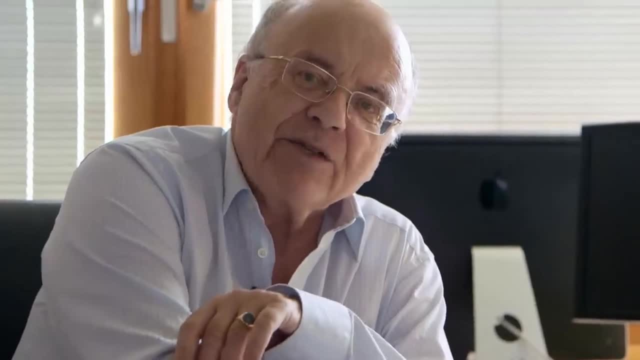 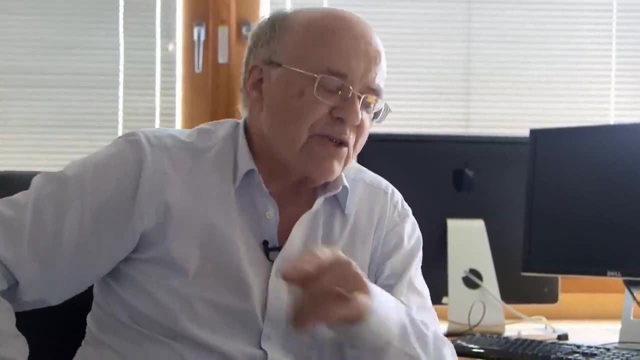 which we've got here are for when m gets down to 0 and when n gets down to 0,, then in the end it will terminate, So long as you feed in positive integers for m and n. Now, as ever, I have done no error checking. 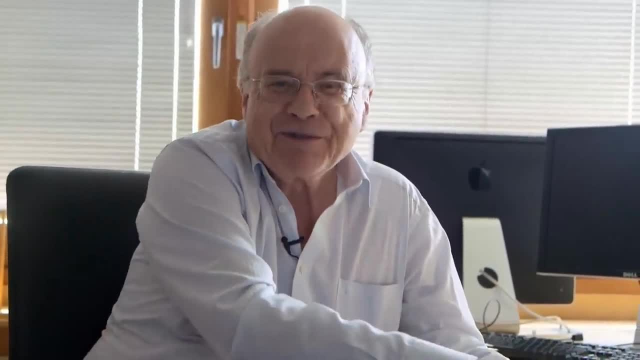 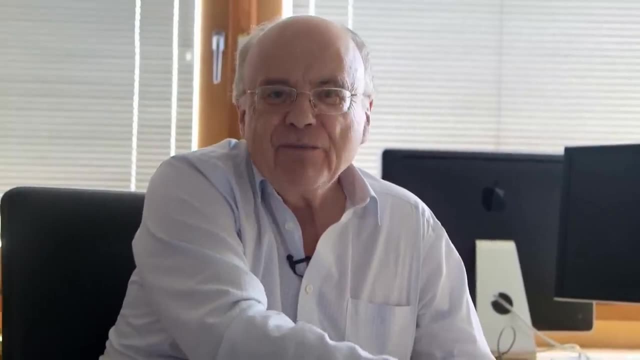 Whatever That's down to you. I want you to concentrate on this. Yeah, If you put negative in numbers in there, boy, are you in for a rough old ride. Yeah, It's got to be positive integers. Zeros are fine. 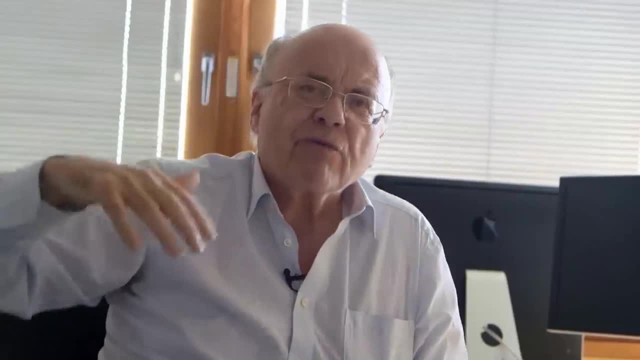 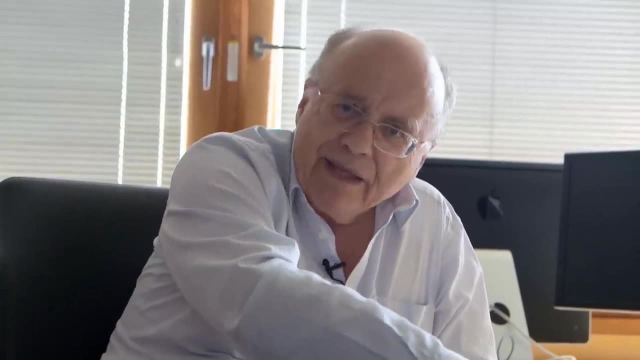 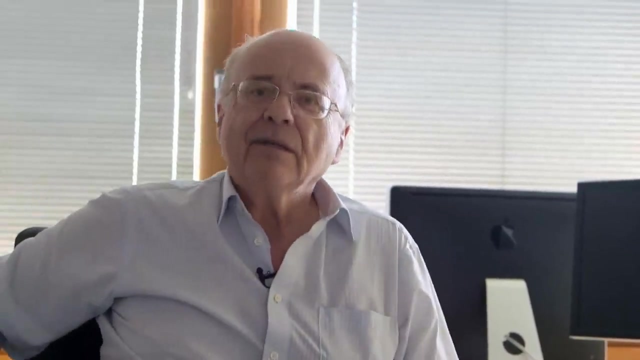 but it must be zero or positive integers. Although this is a huge recursive mess with millions of stack frames, nonetheless, by reasoning and saying that when these values are altered, they always alter downwards, you can convince yourself that this will eventually deliver an answer. 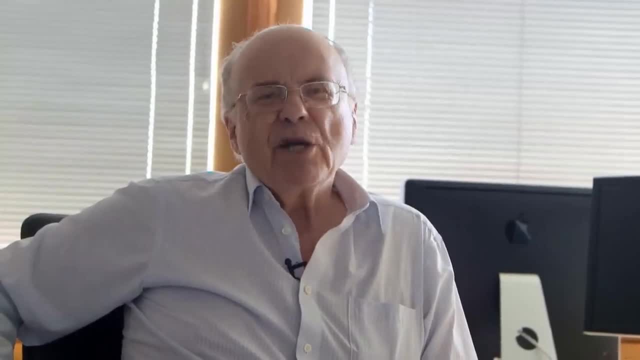 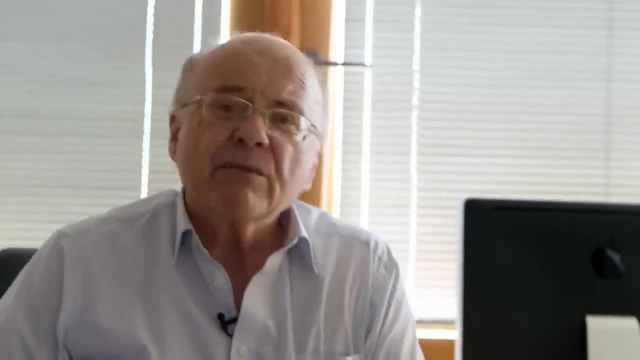 Now the only trouble is in delivering an answer. there may be a huge amount of computation involved, particularly when we get onto this third line and you have to run Ackermann's function in order to work out what an argument to Ackermann's function is going to be. 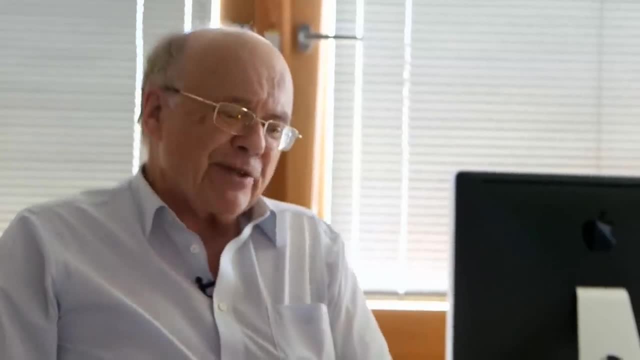 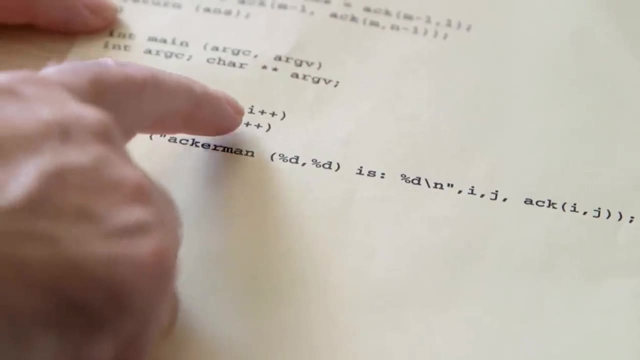 And just to show you how bad this gets, I've set up two nested for loops on i and j, taking i from 0 through to 5, actually, because it's i less than 6, j from 0 through to 5,. 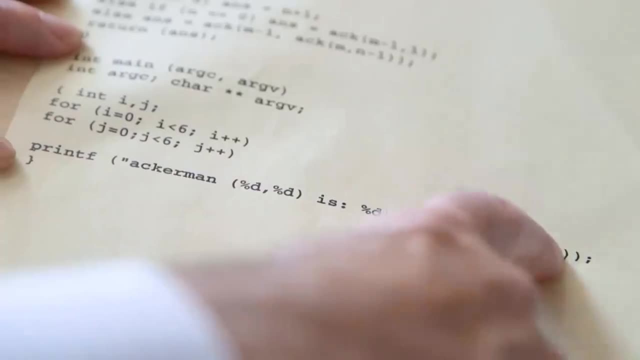 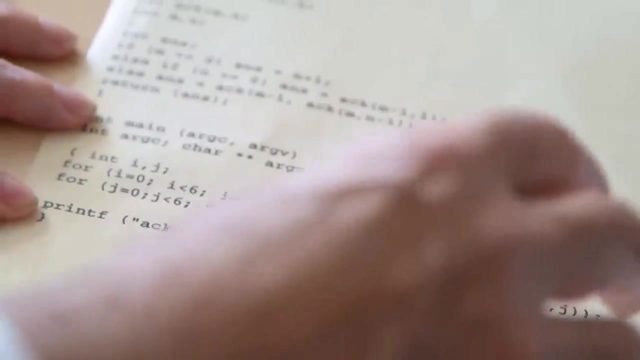 and I call up the Ackermann function as the argument to be printed in the standard piece of text here. So you get things like Ackermann 0,, 0 is whatever, and you call up Ackermann recursively to work it out. So how's that going for you? 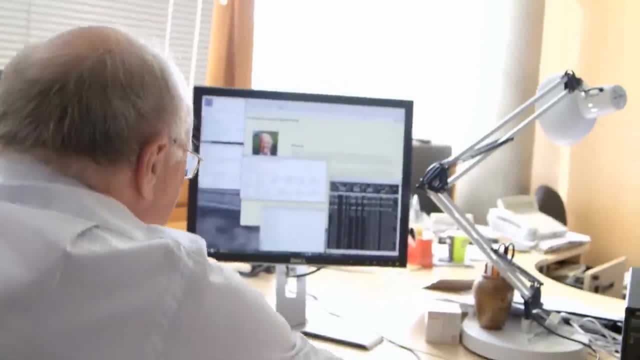 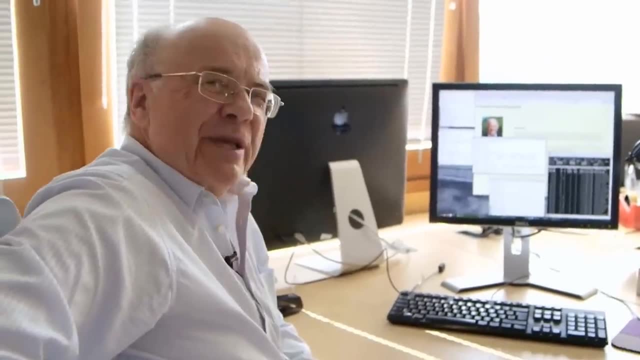 How's that going for me? Well, what Steve and I- Dr Heartbleed, as we now call him- we set this going four weeks ago. nearly now The first few have vanished off the top. You'll be delighted to know. 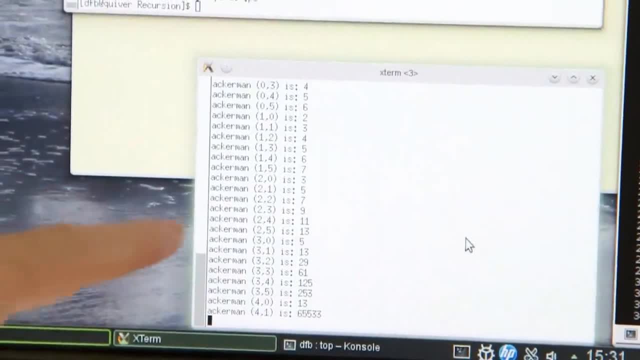 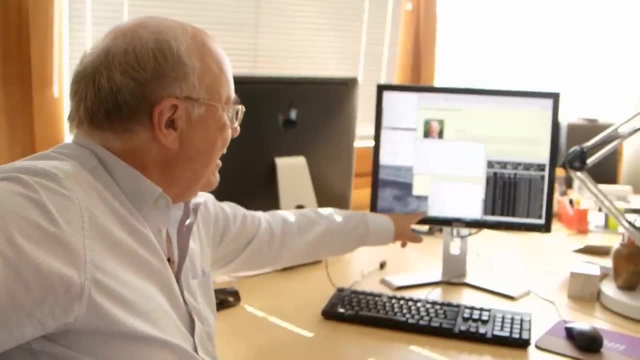 that Ackermann of 0, 3 has a value of 4, that Ackermann of 2, 2 is 7, Ackermann of 3, 2 is 29,. doesn't look too bad. Now, it did have a bit of a gasp for air. 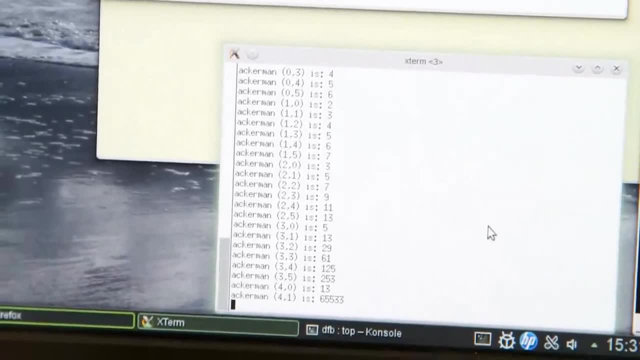 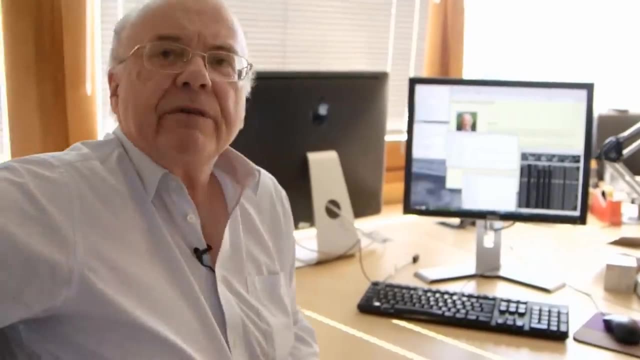 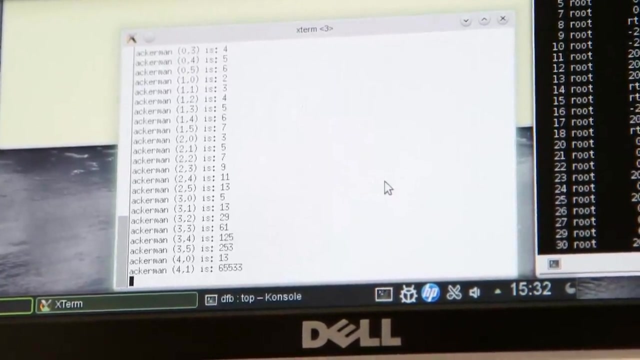 between 4, 0,, which is 13,, and it finally decided that Ackermann 4, 1 was 65,533.. It still took it recursively on this machine three minutes to work out that Ackermann 4, 1. 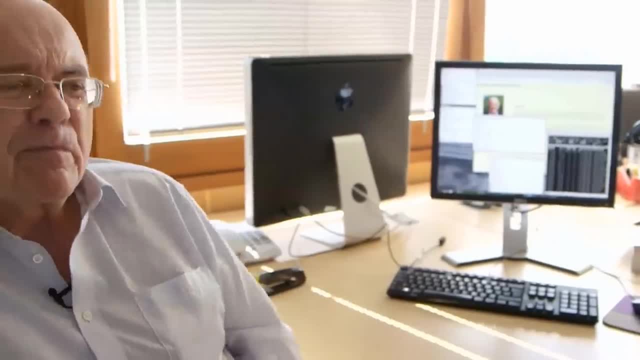 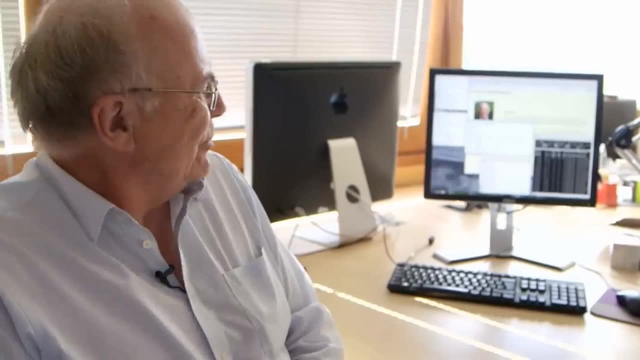 was 65,533.. So this is progress, because this, of course, is a fairly modern quad-core Pentium or whatever it is, running Linux, The previous machine I had when I first tried this about 7 or 8 years ago. 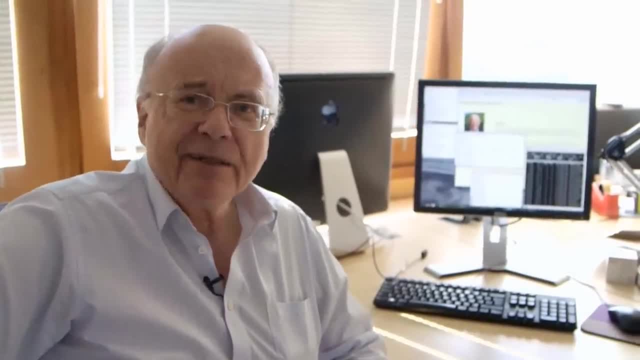 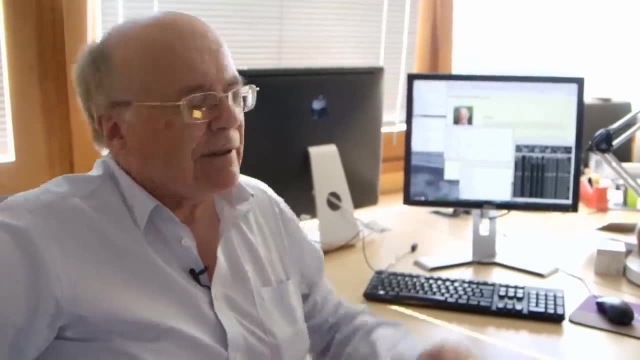 was a venerable son, SparkBlade, And the SparkBlade miracle of its age took 20 minutes to work that out. So 20 minutes, three minutes, we're progressing. And then you know I was looking at this. 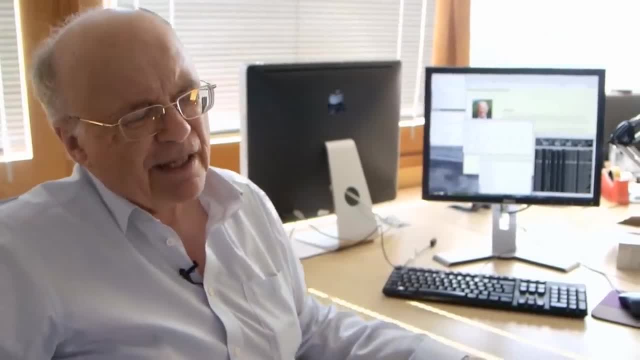 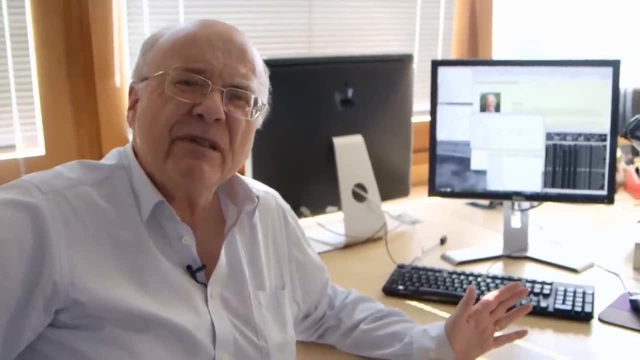 with Steve. we've set the thing going. it's still running and I said, oh, you know, it probably won't be that bad it'll be if it took three minutes to work out something whose answer was 65,533,. 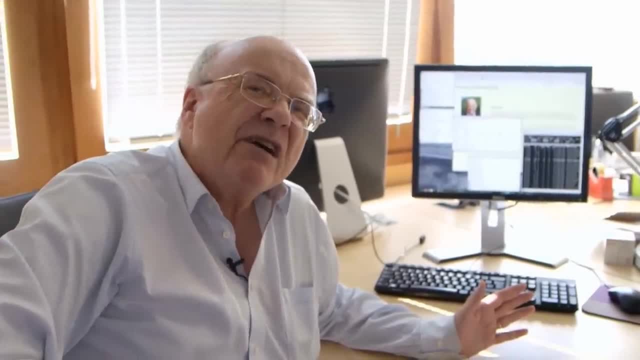 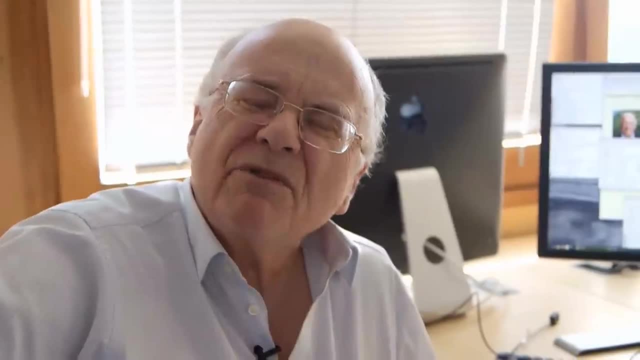 it'll take about maybe 65,000 times three minutes to work the next one out And did a few calculations. yeah, about four months on this machine, something like that, Er no, I looked into it more deeply and reminded myself. 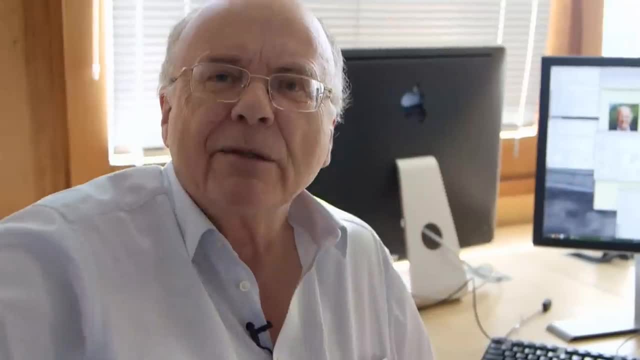 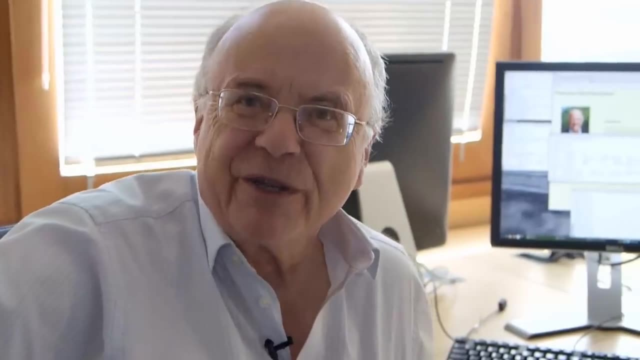 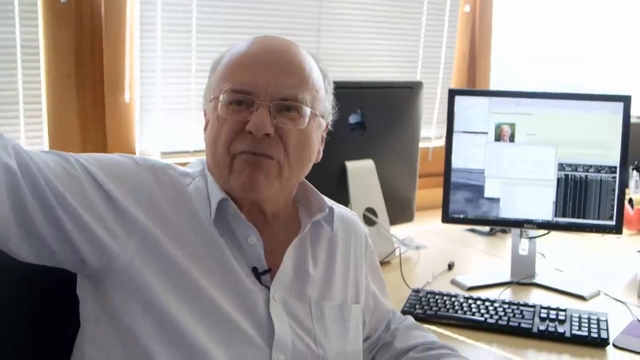 of the appalling properties of the Ackermann function when it starts to build. No, It will take two to the power of 65,533 times three. three minutes per go: it will take three times two to the 65,533 minutes to work. 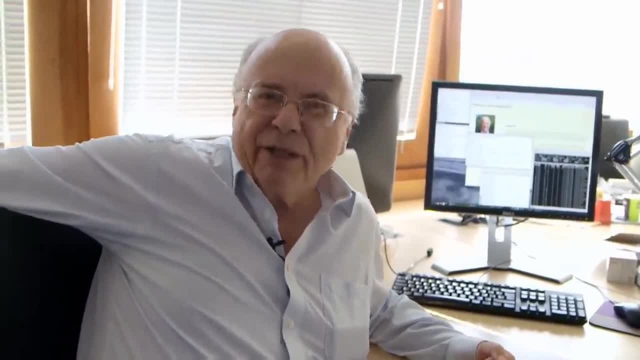 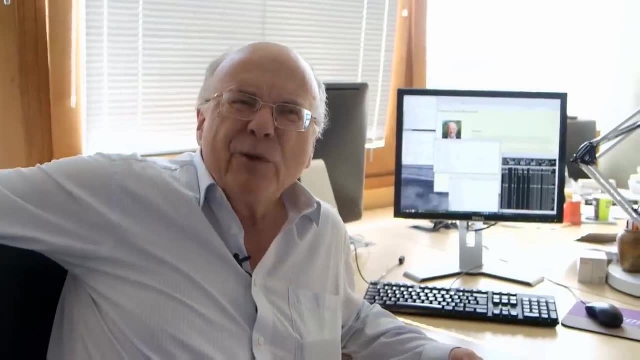 out that value. That is unimaginably huge. It's no good saying it's astronomical, It's way beyond astronomical. The number of particles, I think, including all dark matter, isn't more than about two to the three hundred, something like that. 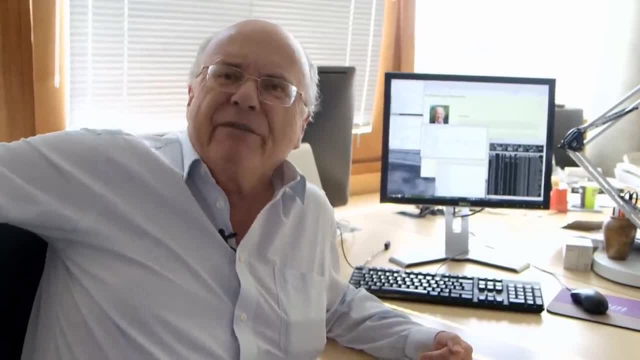 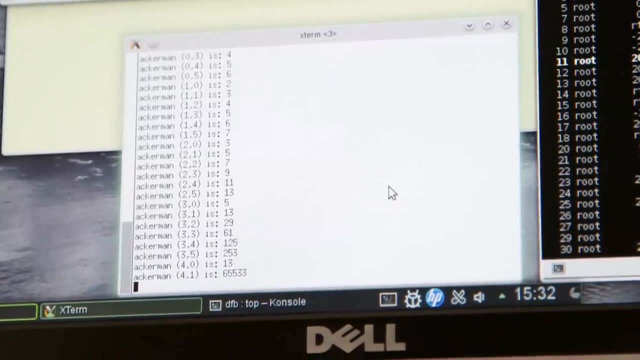 The number of seconds since the Big Bang is probably about two to the five hundred or six hundred at most, not two to the power of 65,533. But what's going to happen eventually? Two to the power, 65,533 is such a. 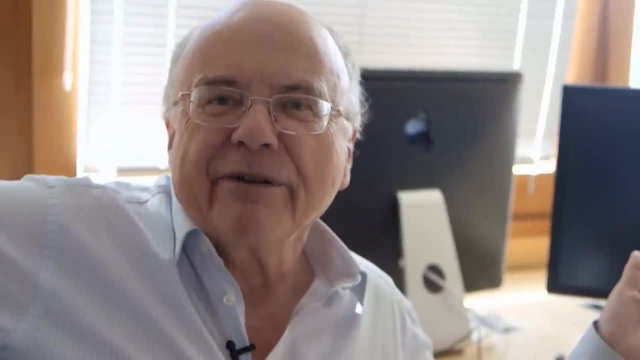 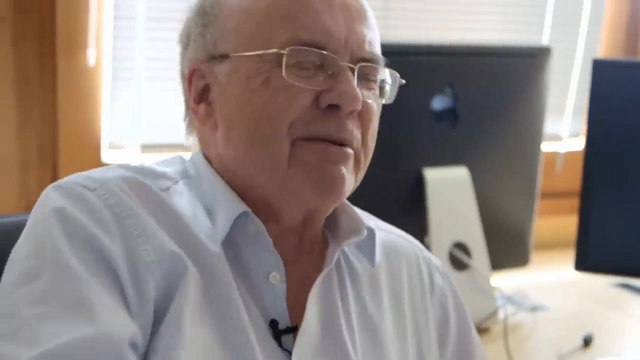 big number. So we're going to start getting wrong answers. We'll either get overflow happening or perhaps, if integer overflow isn't signalled to us, you know, integer numbers sometimes tend to roll over the top and go negative. So 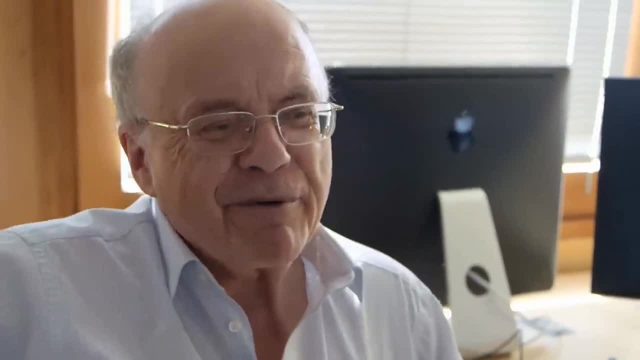 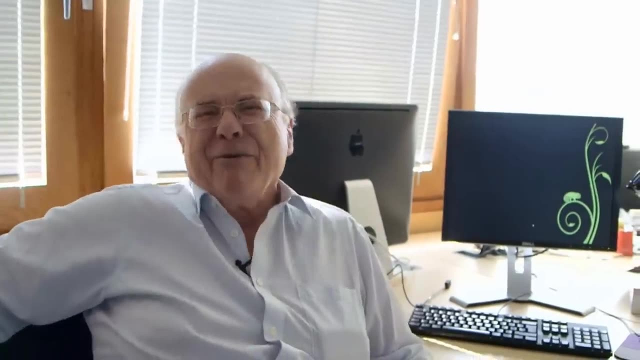 who knows what will happen. I'll probably stop this off now, when we've made this video, because, frankly, I have not. I don't think I'm going to survive for two, to the power of 65,533 minutes multiplied by three. 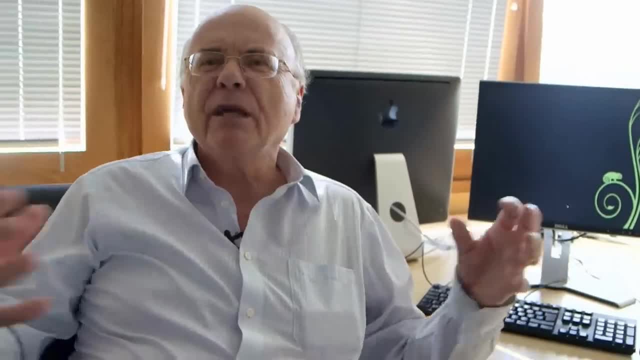 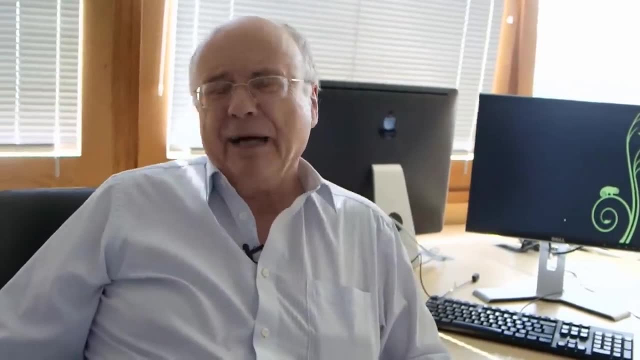 for this to come to an end. I think the astronomers will probably say the big crunch when the universe all gets down to a dot again. Even that is probably going to happen in about another two to the power few hundred. This sort of behaviour is often called super-exponential. 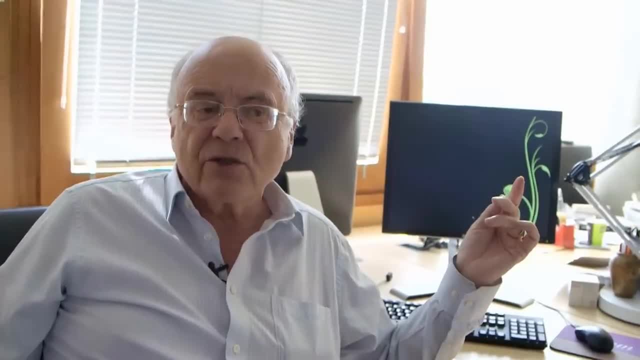 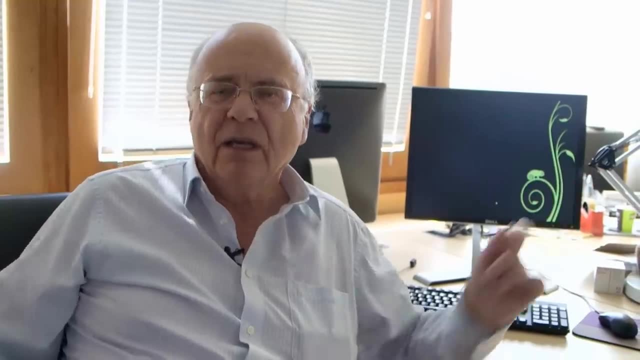 One of the ways of indicating that a function probably has to be done recursively and can't be done in for loops is when it starts behaving super-exponentially, Not just like n to the power n, which will be exponential, but n to the power of. 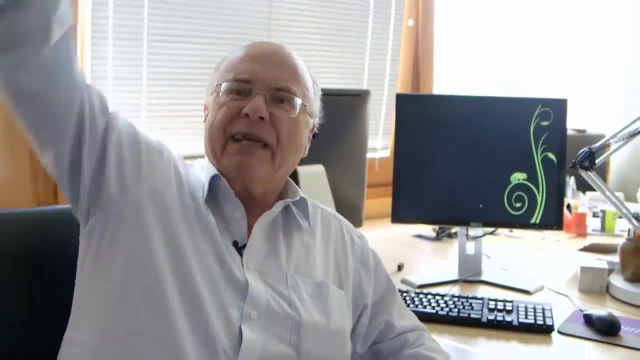 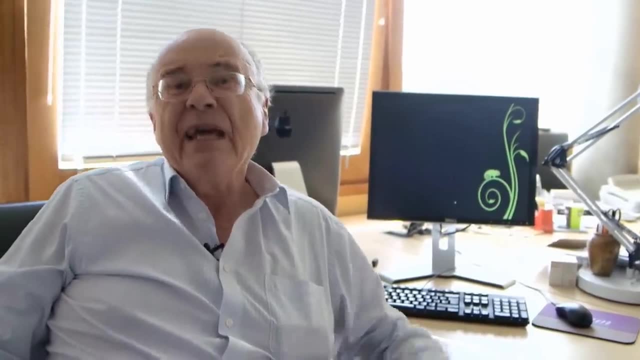 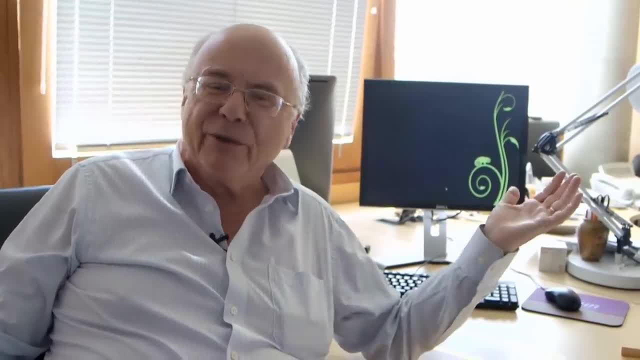 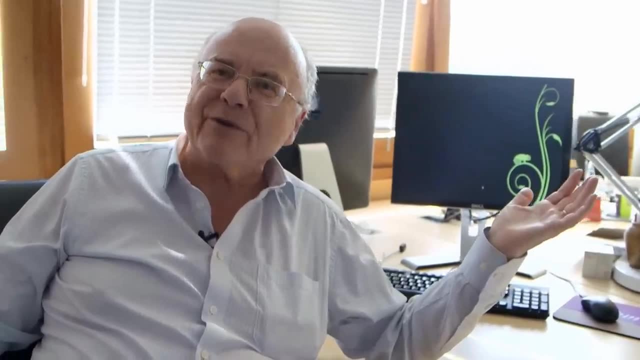 surely you can do anything in for loops? what do you have to do totally recursively? Somebody's picked up, I think, one of those numbers I don't know much about, really big ones called Googles and Googleplexes, but they've been covered in.